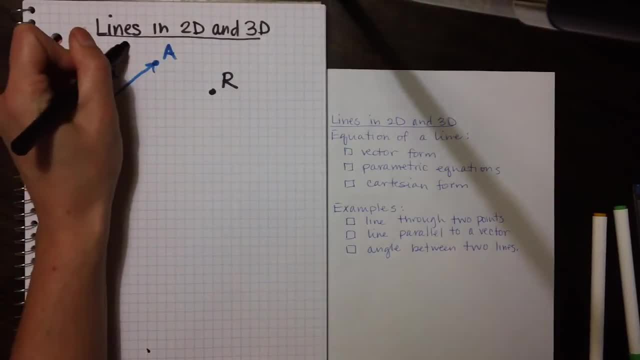 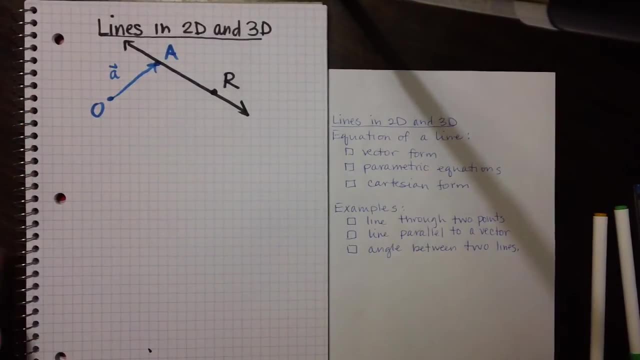 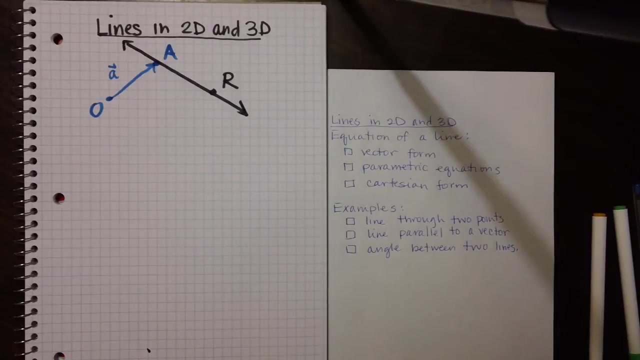 other point, R. I know that two points define a line and I know that if I have the coordinates of A and R, I can write the equation of the line that goes through them. And the form that you usually write the equation of a line in is called Cartesian form. Today we're going to learn the vector. 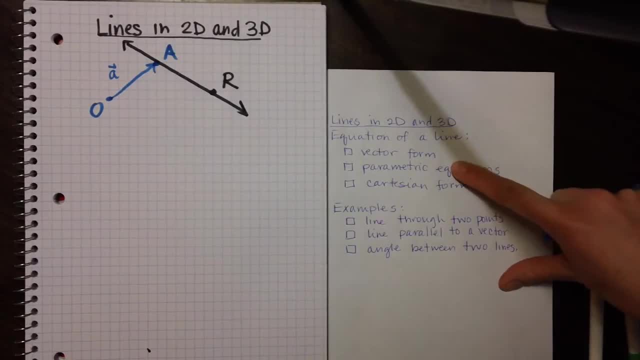 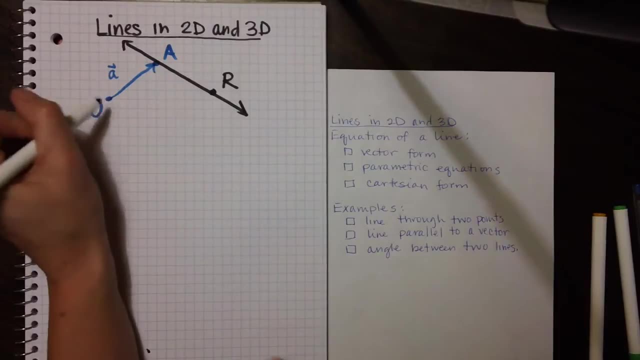 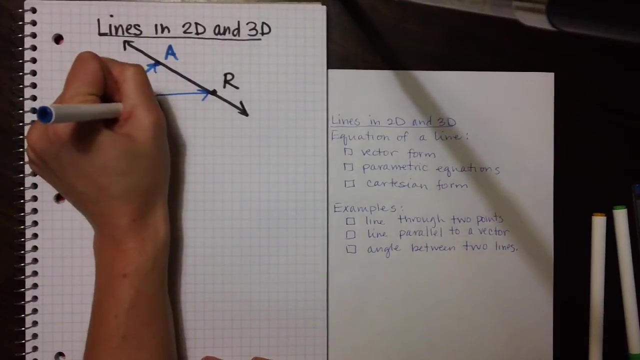 equation of a line. We're going to see how to break that up into parametric equations of the line and how to convert those into Cartesian form, which is the familiar form of a line. So I can also write a position vector from the origin to point R, vector OR, and I'm going to call that vector little r. 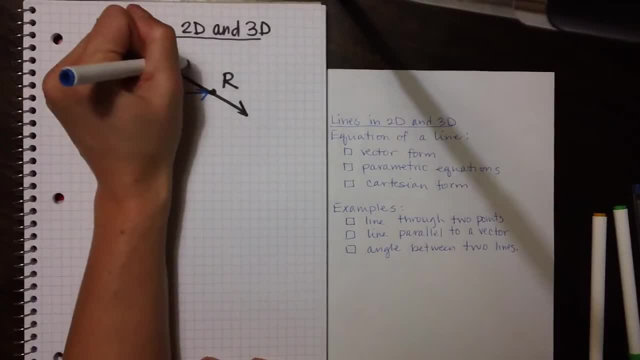 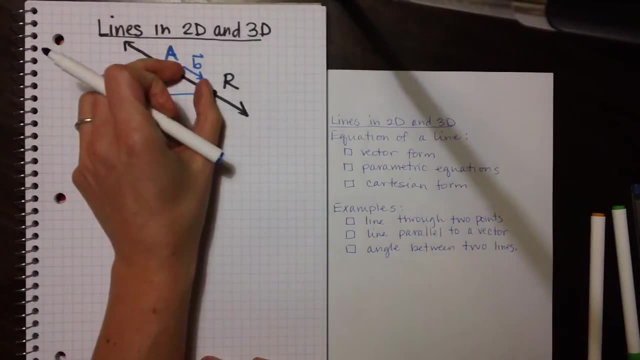 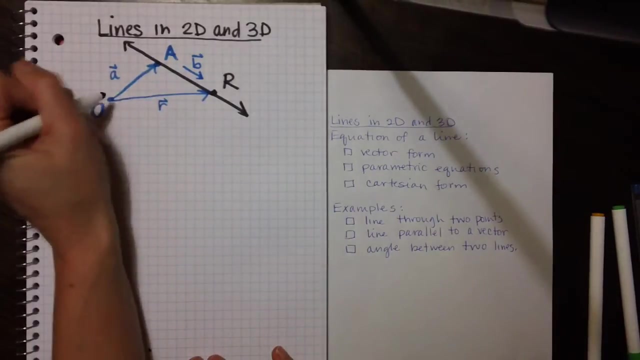 If I know the direction that my line is pointing in, or I can say that my line itself is parallel to some vector B, but obviously it's not the same magnitude because it's a line, so its magnitude is infinite. All right, so again, R is the position vector from the origin to any point on the line. 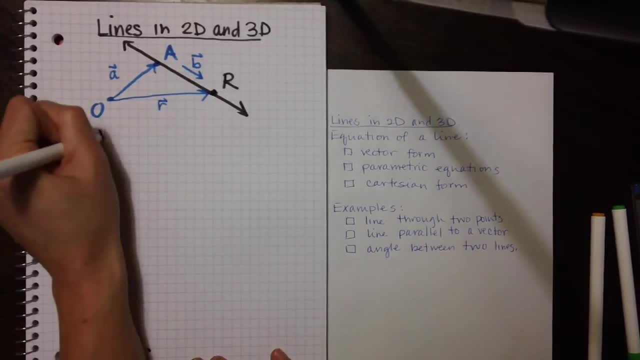 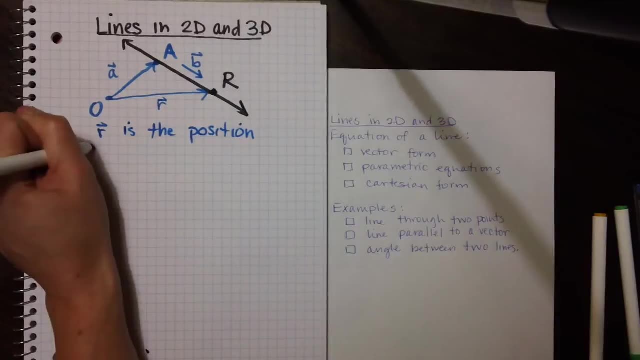 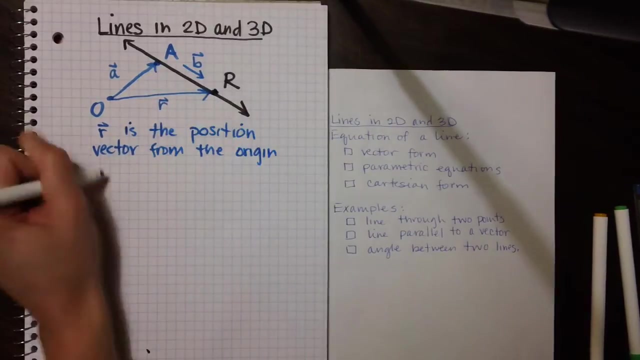 in the point x, and I'm just naming this other point R. deshalb � admittance Exceptions we're using uh... A i do e c o y r d i u s s d t h x s r x i e l d s 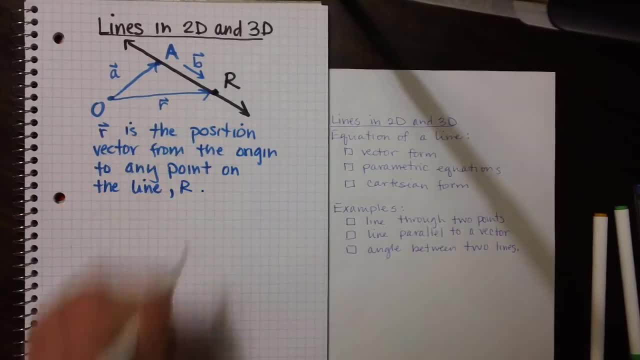 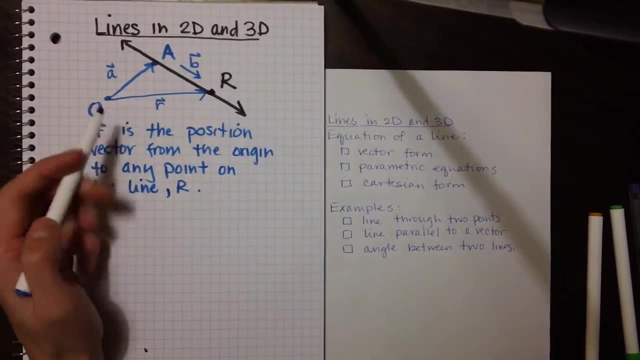 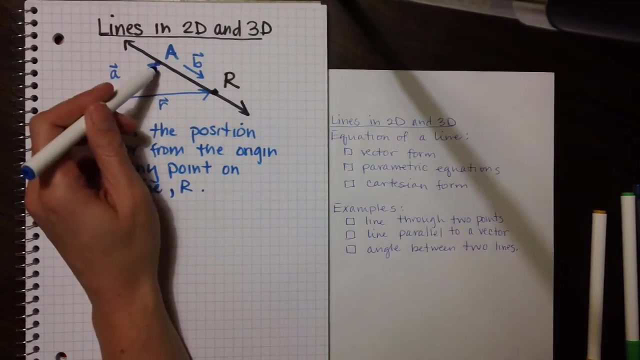 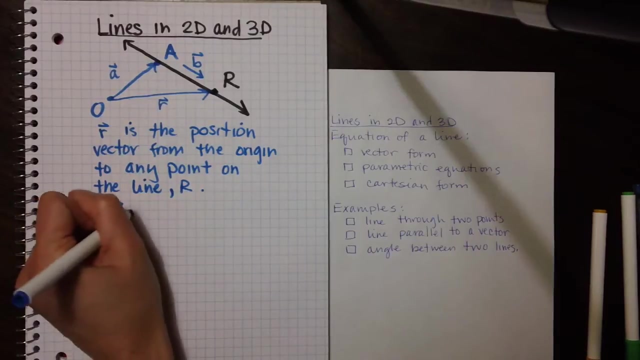 d cy se point non s t r сы e t. I know about vectors to write an equation for this position, vector R. I know that vector OA plus vector AR is equal to this position. vector R. OA plus AR is equal to OR and OR. 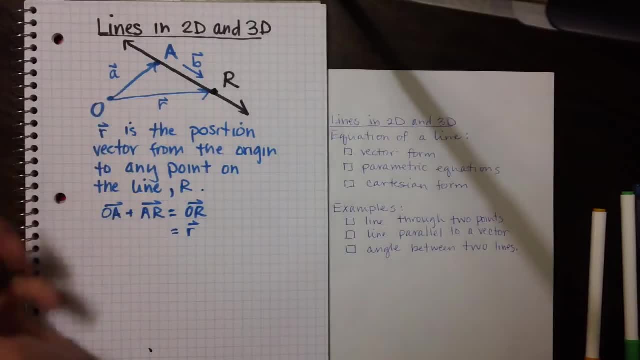 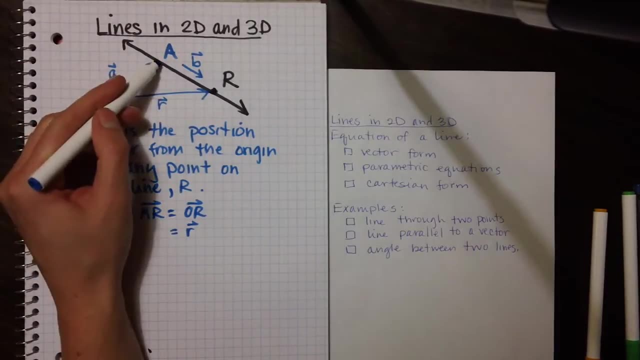 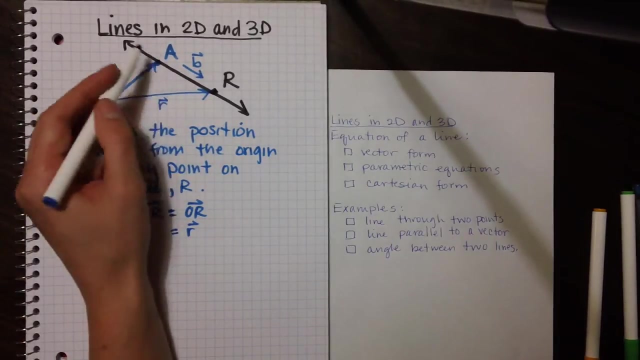 is my position. vector R OA is this little vector A from the origin to point A, And vector AR. I don't know how long it is, but I know what direction it's going And because I know that vector AR is parallel to vector B, I know that vector AR. 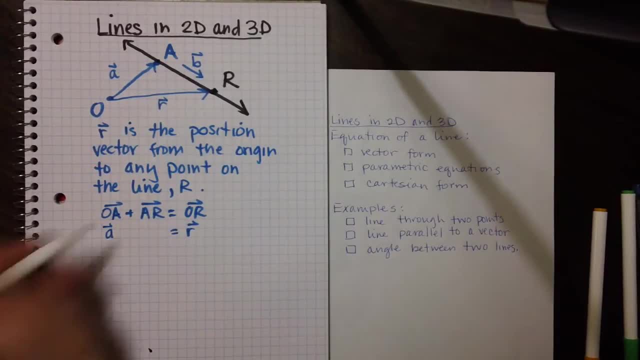 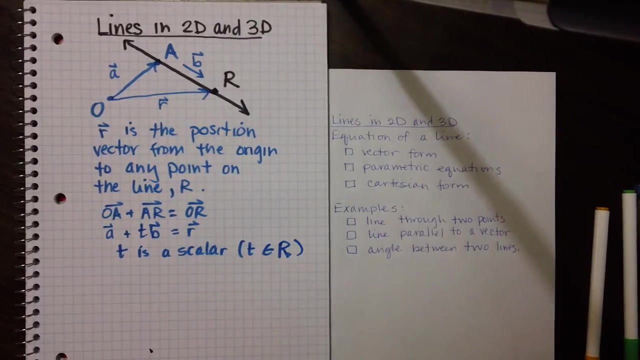 has to be a scalar multiple of vector B. So instead of AR, I'm to write a scalar multiple of vector b, and the scalar I'm going to use is t. So t is a scalar. It's just some real number. so t is an element of the set of all real numbers. 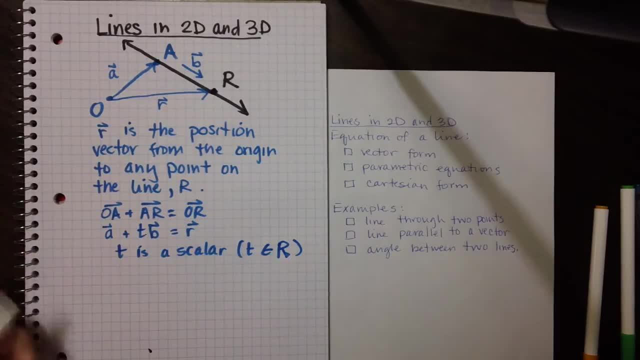 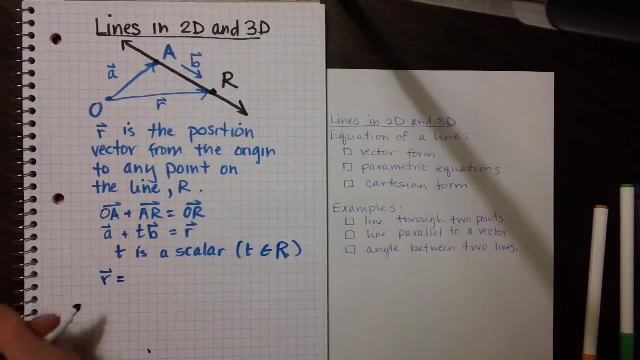 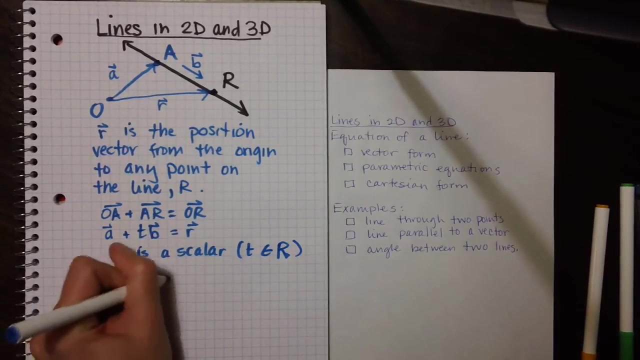 All right, so this is the vector form of the equation of a line. The position vector from the origin to any point on the line is equal to the position vector from the origin to some other point on the line. this is usually a reference point or a given point plus some scalar parameter. 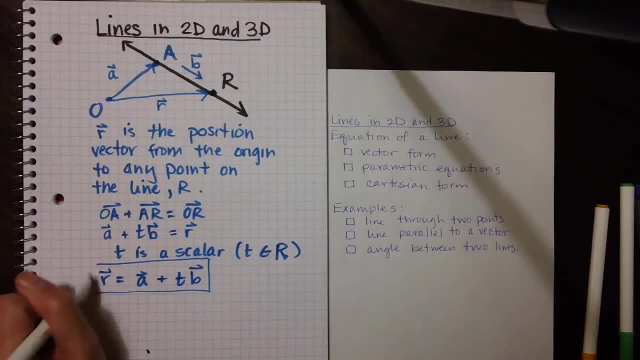 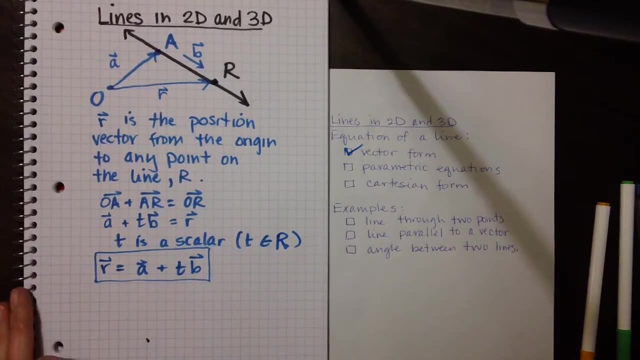 times the direction vector b Vector. equation of a line. If I think about the components of the vectors r, a and b, if it's in two dimensions, then r would have an x component and also a y component, the same with a and the same with b. 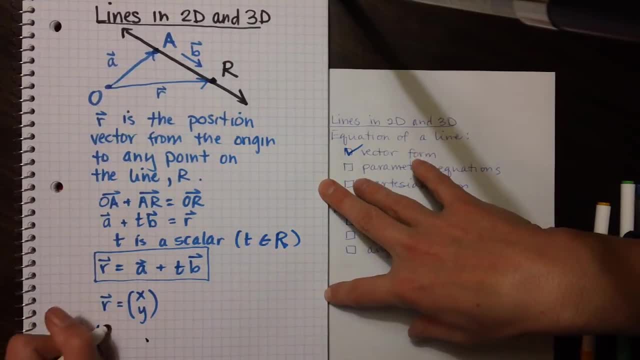 So if I write this out like this, I could say: the x and y coordinates of point r is equal to the x component of vector a, which I'll call a sub x, and then this is the y component of vector a, a sub y plus t. 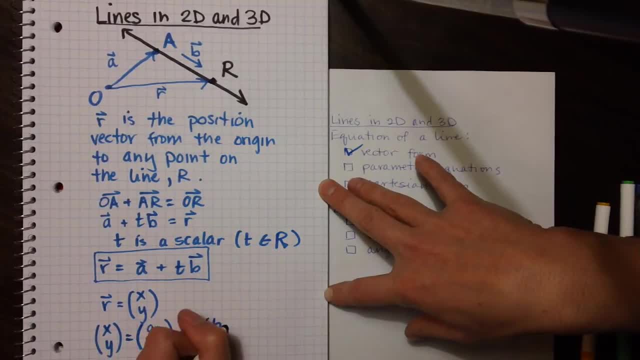 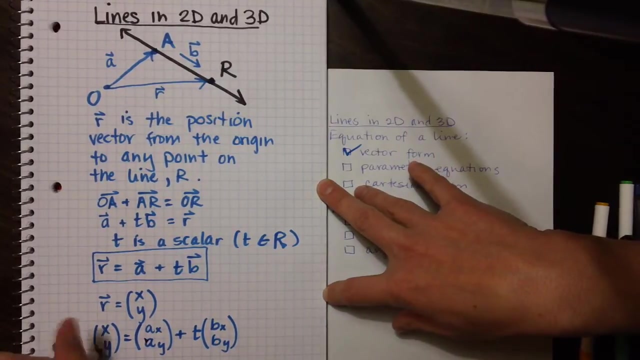 ここ이 계산 세 �с, which is the y component of vector b. Now, if I take my scalar parameter times, the x component of the direction vector b and the x component of direction vector y, if I write my vector equation of a line in component form, I can split it into two. 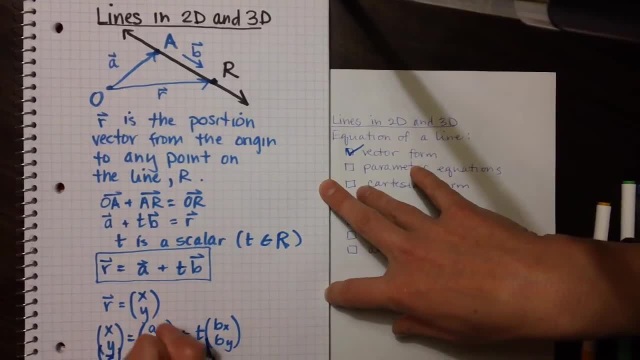 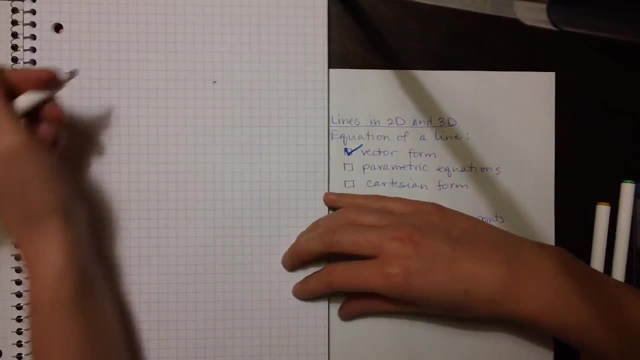 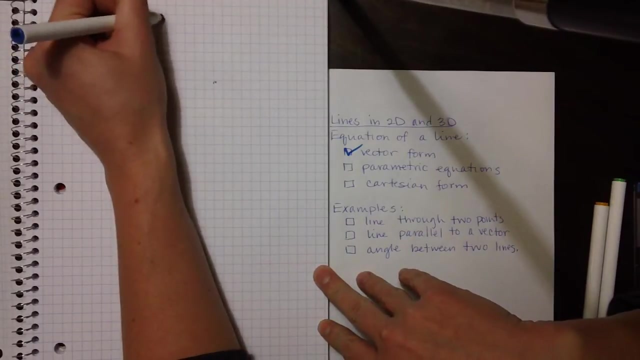 equations: my x equation and my y equation. If I was in three dimensions, I would have, of course, a z down here, So I would just have three components, three equations where I'd have: X is equal to the X component of A plus T. 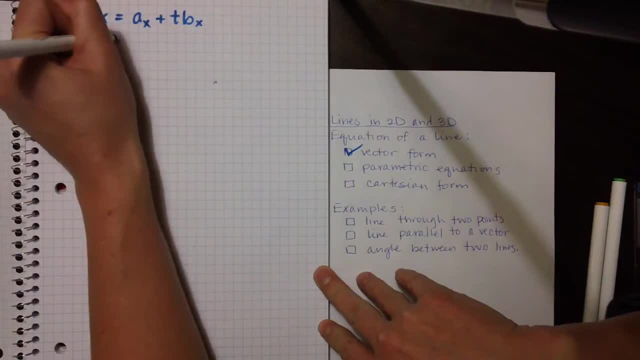 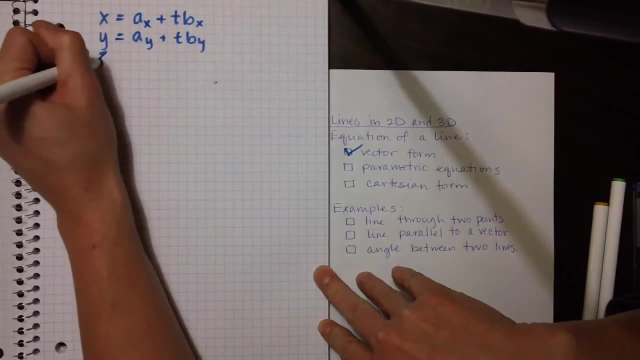 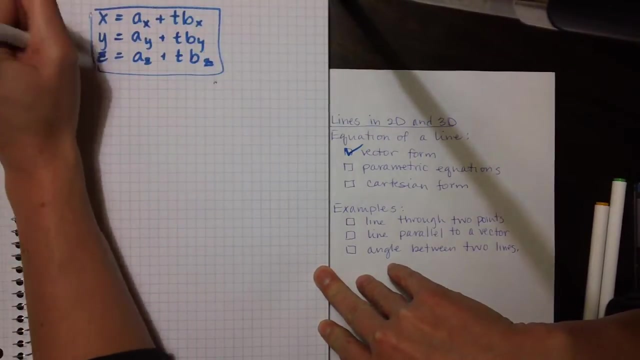 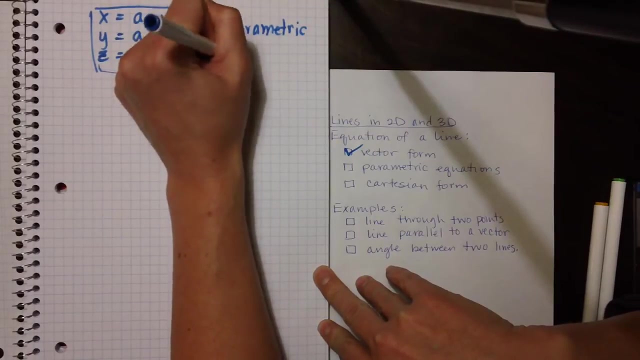 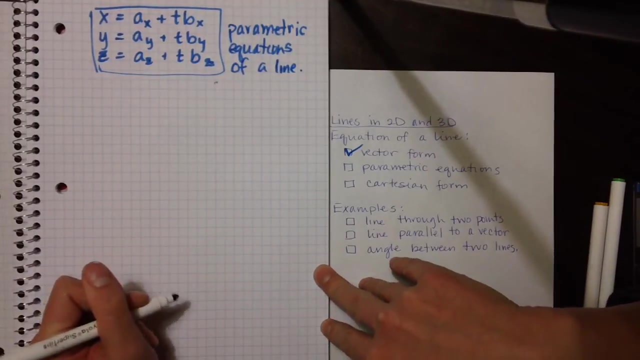 times X, component of B, and so on, and these are my parametric equations of the line. so again, these are the parametric equations of the line. I can convert my parametric equations into a Cartesian equation, which is the standard. choose the perfect reasszetarea. 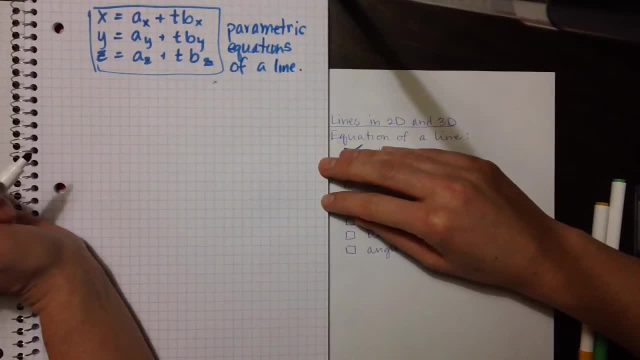 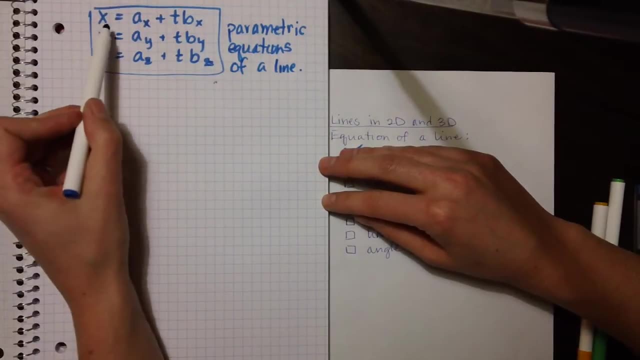 equation of a line that you're used to looking at and working with by eliminating the parameter. So I'm just going to do this in two dimensions, just for simplicity's sake. Actually, no, I'll do it in three. So I want to solve each of my parametric equations for my parameter t, Then I 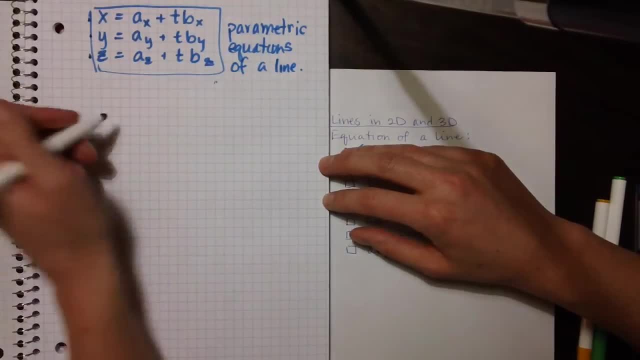 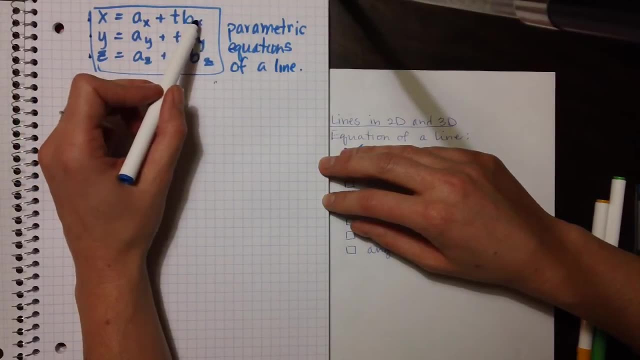 can set them equal to each other, All right. so the first one: if I solve, x equals the x component of a plus t times the x component of b for t. I'm going to get x minus. just stay on it, thank you. 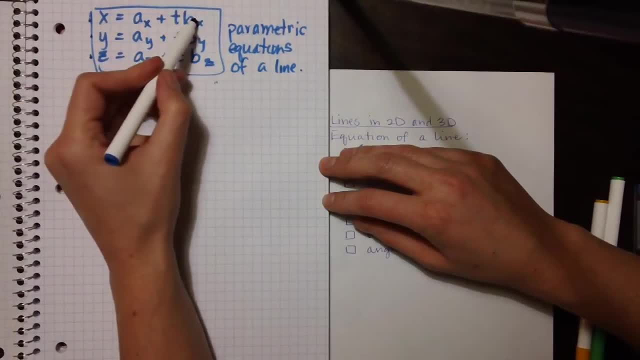 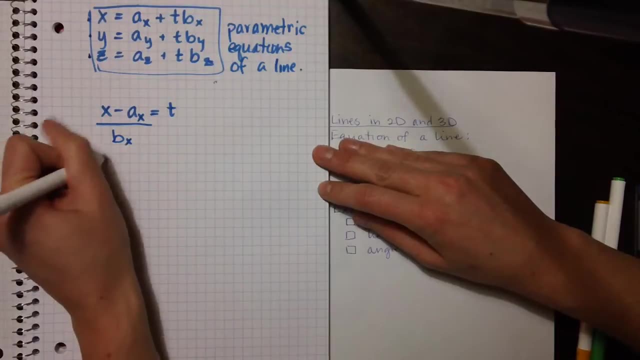 a sub x is equal to t times b sub x. So if I want to solve for t, I just divide by b, like so, And I could do the same for the other equations. It would be: y minus a sub y over b sub y is equal. 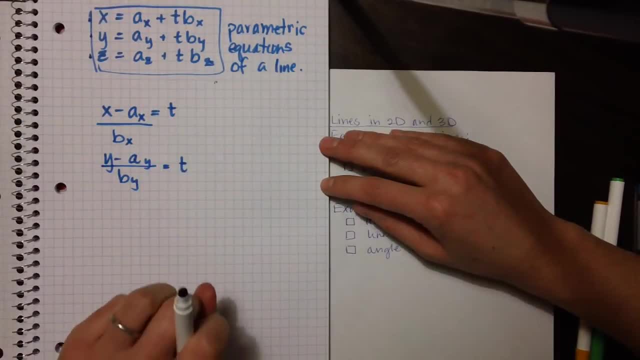 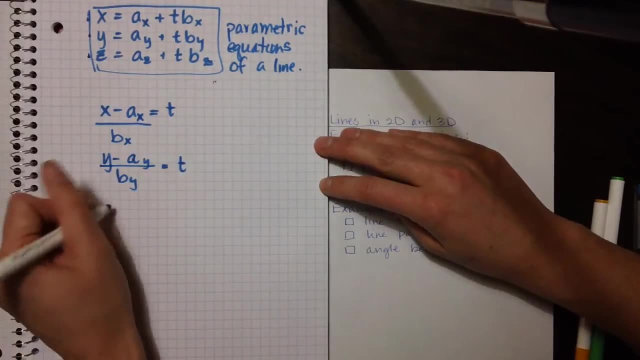 to t. I changed my mind. I'm just going to do this in two dimensions. So for a line in two dimensions, I can get the Cartesian form of the equation by setting t equal to t And I'll have x minus a sub x over b sub x. 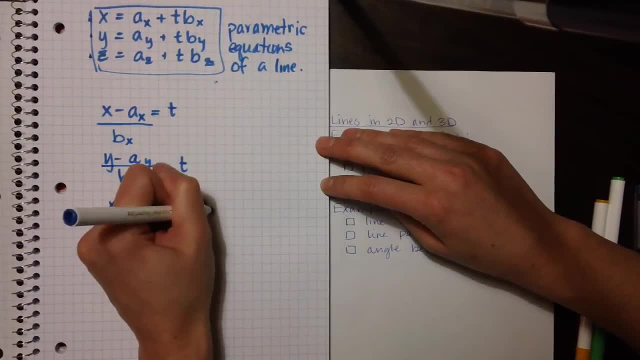 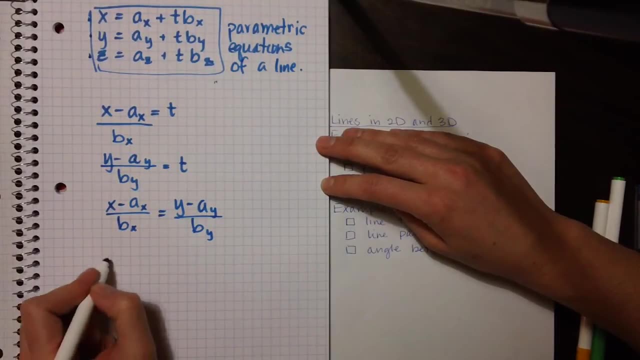 is equal to y minus a sub y over b sub y. If I rearrange this equation, I can get it into the standard form, which is some coefficient a, x plus some coefficient b. y equals c, right? Or I could put it into y equals mx plus b, which is a different b than this.